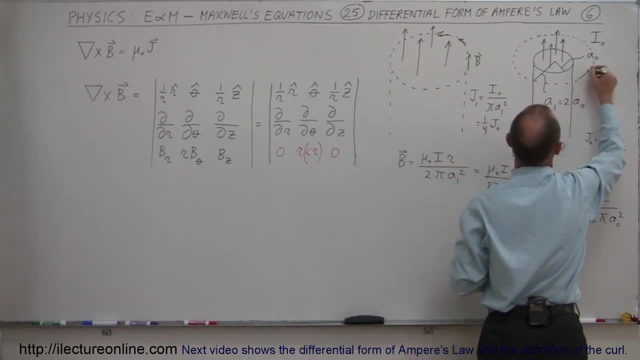 right. So it's a function of theta. So again, we want to find the B-field here at this region. B-field is equal to question mark is equal to question mark. That's what we're trying to find out. So we're going to simulate as if the same current is spread over a wider region and then 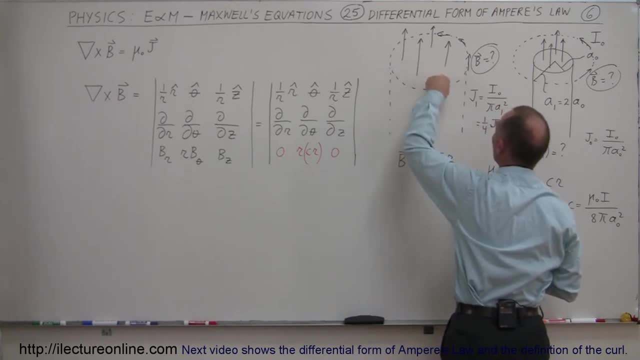 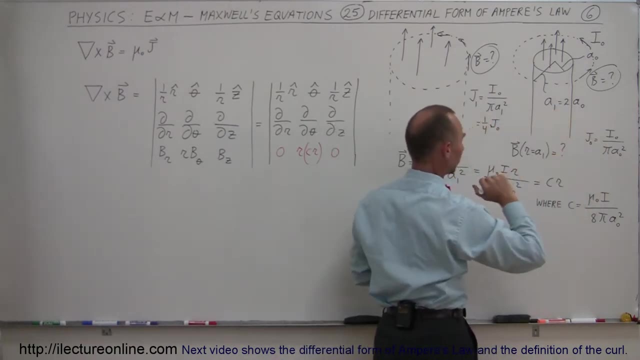 we're going to find the B-field inside this region, all the way out to the edge of that region, using this equation rather than the B-field. So we're going to simulate as if the same current rather than this: Oh where's the equation? I would not want to use. I didn't write it down, So 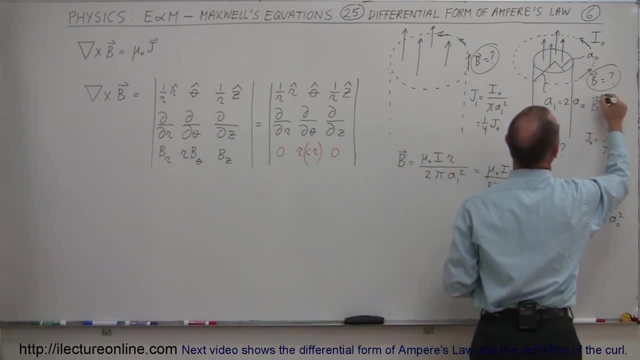 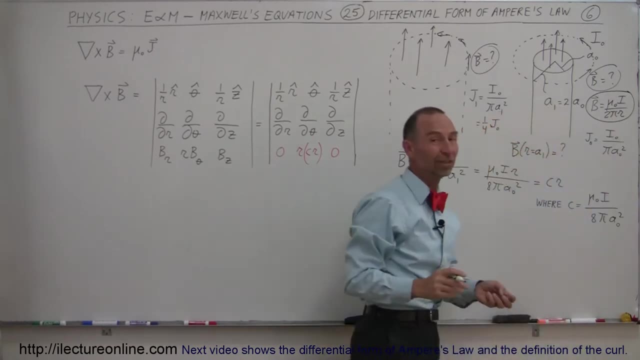 let me write it down. So normally, outside the region, we know that the B-field is equal to mu sub naught times i, divided by 2 pi times the radius. So this is the equation you find by using the integral form of the of the of Ampere's law. Now we want to use the differential form, So we: 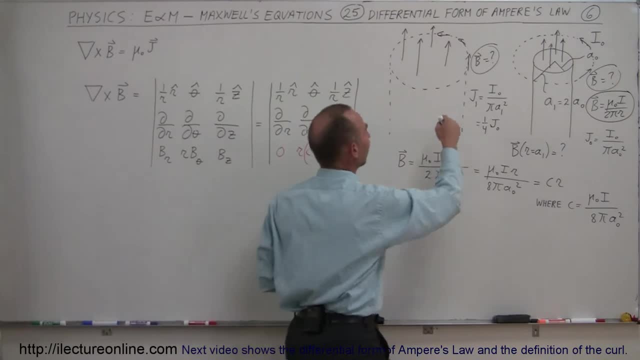 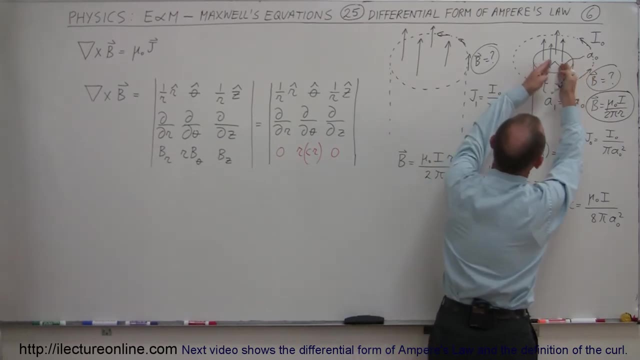 want to take the curl, But to do that we're going to use the inside form of the equation, In other words, the equation as it's valid where the current is happening. and since there's no current out there, we're simply going to simulate as if the current is. 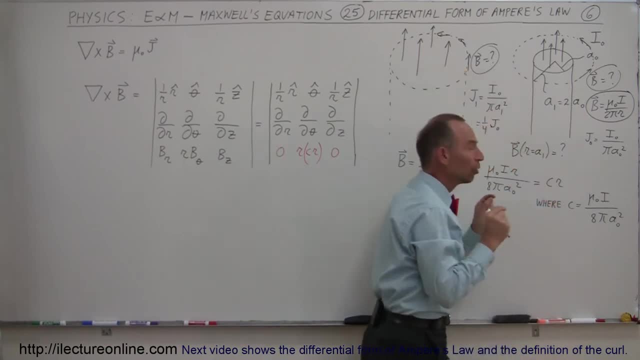 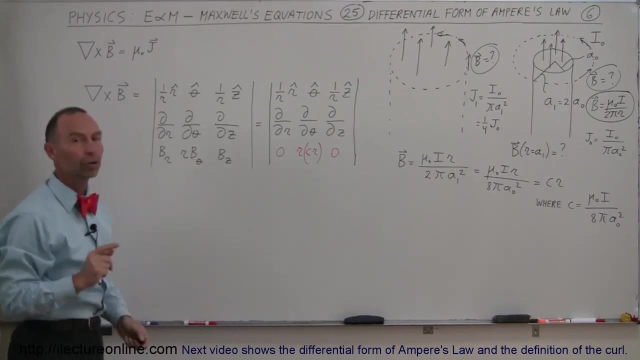 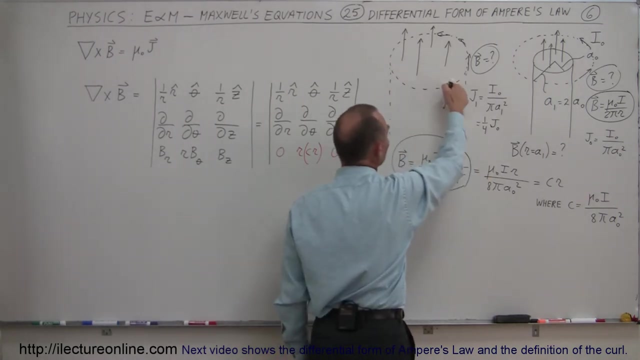 always spread out. to this point, right here And at the very edge. right there, the two equations should converge And that allows you to use the differential form of Ampere's law and allows you to find the curl. So we know now that this is the equation of the B-field inside this current 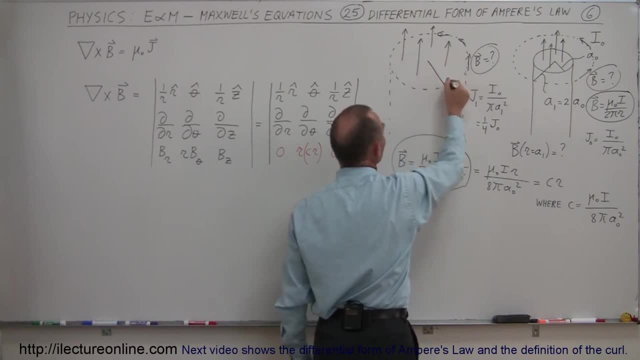 region right there, all the way from the center, all the way out to the very edge, And of course this now is a1, which is 2 times a sub naught. So we want to find it At a distance that's twice the radius of this inside region where the current is happening. 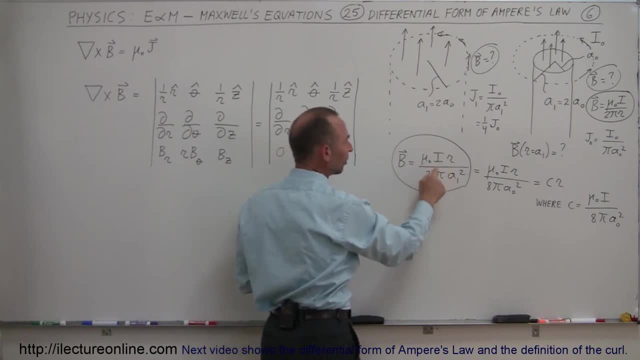 So the equation then becomes: mu sub naught i times r divided by 2 pi a sub 1 squared, And since a sub 1 is twice a sub 0, this then becomes mu sub naught i r over 8 pi a sub naught squared because 2. 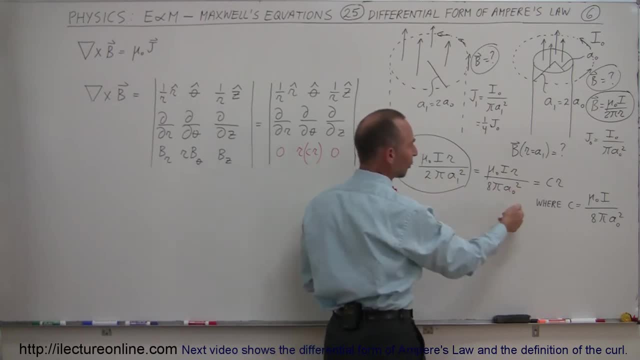 squared is 4, and 4 times 2 is 8, right here. And of course then we're going to simulate, not simulate, but we're going to make the equation easier to read by simply taking this portion of the equation, call it a constant and multiply times r. So c is simply mu sub naught, i divided by 8, pi a sub naught. 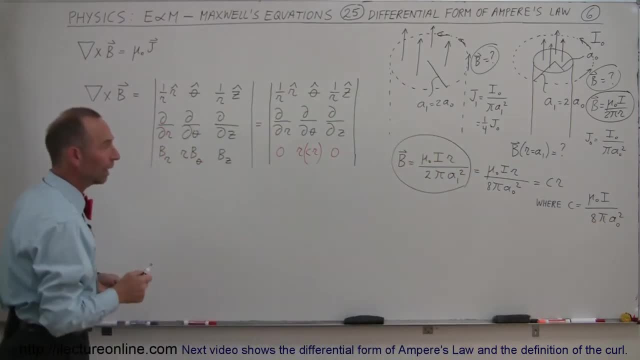 squared. Now we can use that in the curl equation and then we can show you how this form actually works. So this is what we call the curl of a vector B. In this case, vector B represents the magnetic field in cylindrical coordinates And then, of course, the B-field in the r direction. 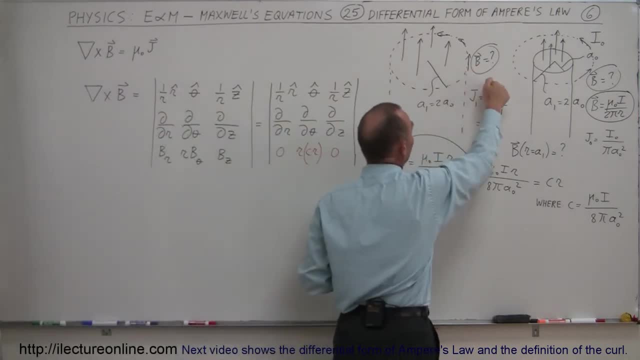 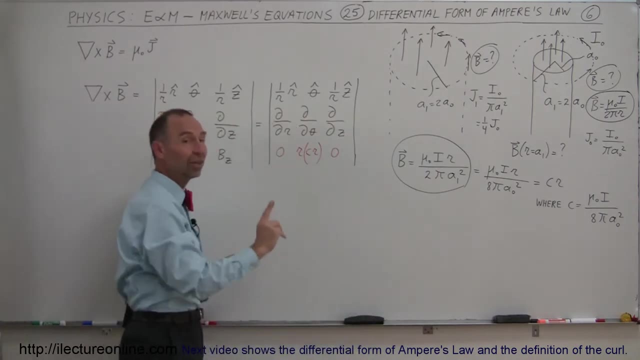 the radial outward direction is 0, because there's no B-field out in this direction, It's only along here, the curve of this circle. so it's zero in the radial direction. it's zero in the z direction. there's no b field going directly up, there's only b field going around the circle, and so that has. 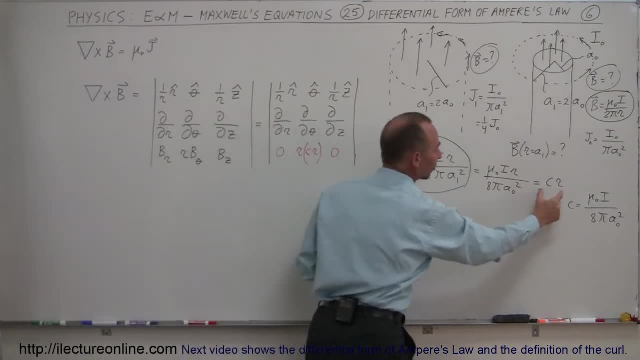 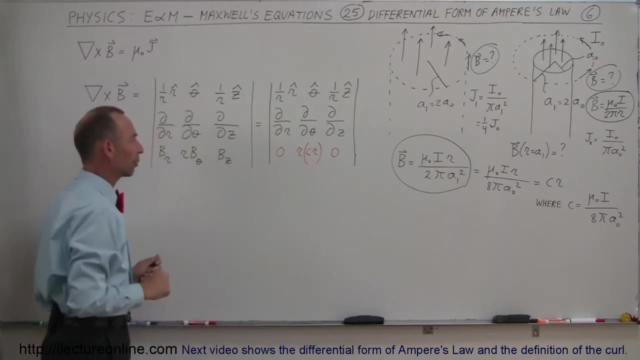 to then this. then c r came from this right here, c r, which represents the b field inside the kernel region, and we have to multiply times r. this comes from the equation, so we end up with c? r squared. If we now take the curl of this, we get the following: so we take 1 over r times the. 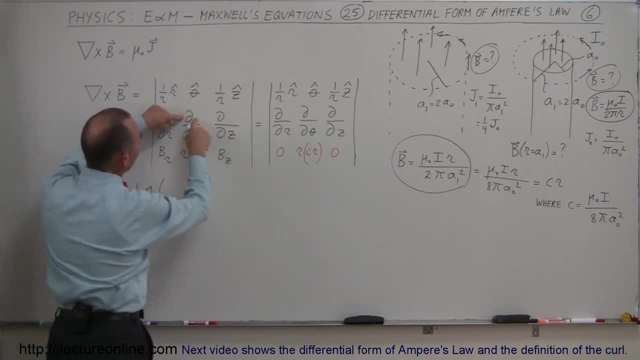 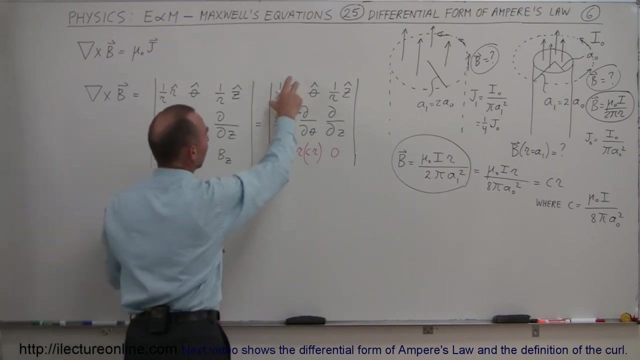 unit vector in the r direction times the partial derivative of theta of b sub z, so the partial with respect to theta of b sub z. oh, instead of b sub z, I might as well write what b sub z is. makes it easier because I already have it there. so here we take this: times the partial of zero. 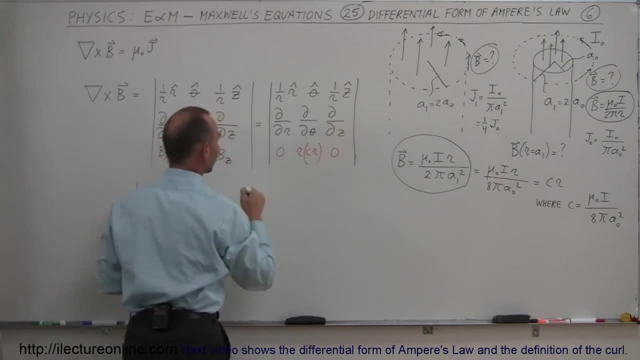 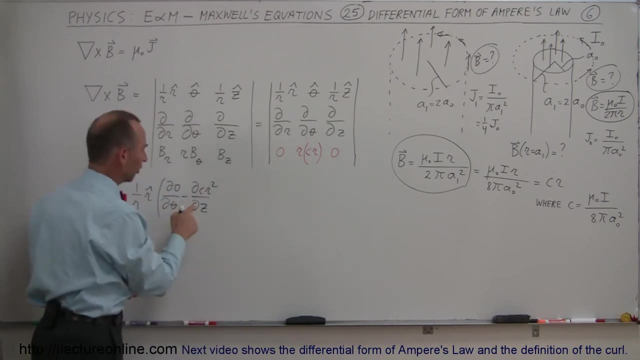 minus the partial with respect to z of this quantity right here. so the partial with respect to z of c r squared. Now, of course, since we take the derivative with respect to z, anything that's not a z is a constant. so here: 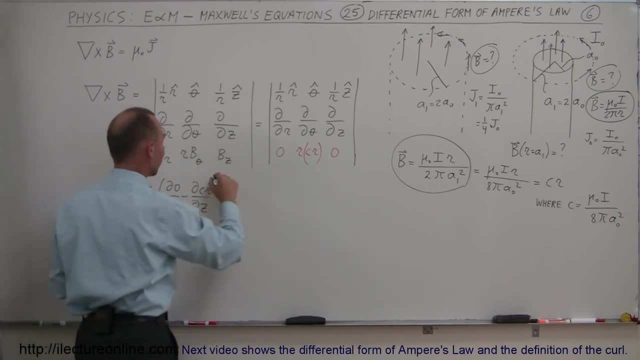 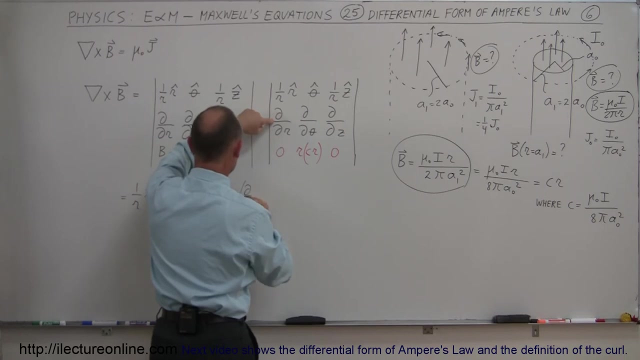 we're taking the partial derivative of a constant, which means it will be zero, Okay, minus, because we alternate signs: plus, minus. plus minus theta hat, that means the unit vector in the theta direction times the partial with respect to r of zero. the partial with respect to r of zero, minus. 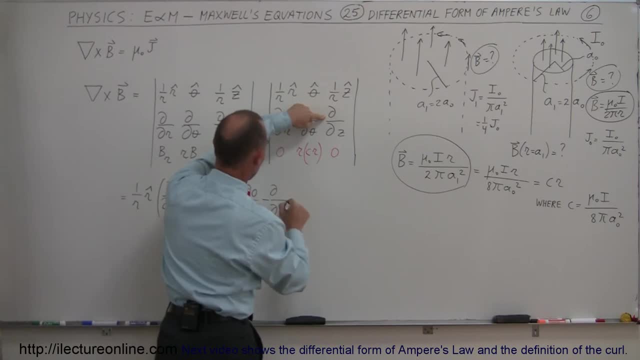 the partial with respect to z of zero. So what you do here is, since you're taking this unit vector, you cross out this column, you cross out this row, you're left with these four elements, and this times this minus, this times this that's. 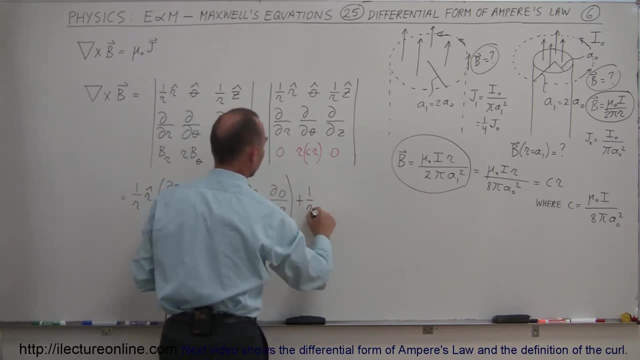 how you get that. and finally, plus one over r times the z unit vector times. so now we use this right here, and then you cross out this column and this row, you take these four elements, so it's this times this minus, this times this. actually it's not a multiplication, you're actually taking. 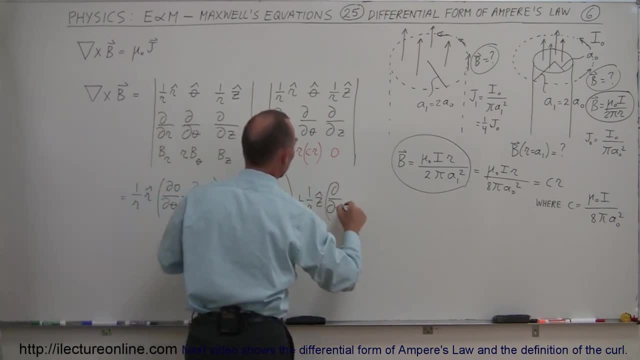 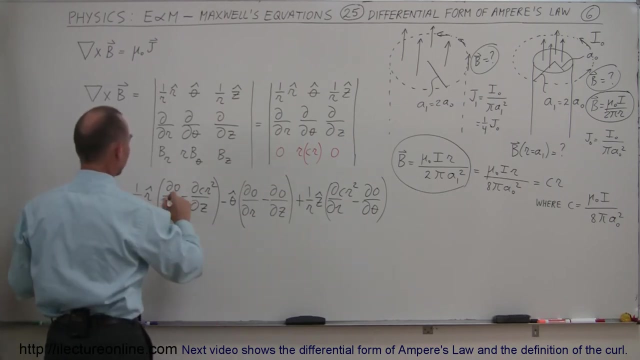 the partial derivative. so it's the partial with respect to r of c, r squared minus. and then we take the partial with respect to theta of zero. Now you realize, when you do this, that every term except one becomes zero. so the partial of zero is: 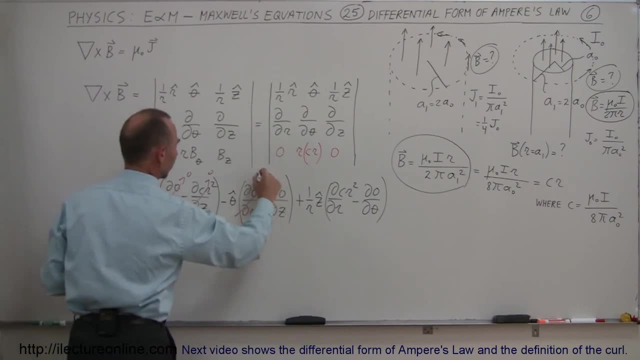 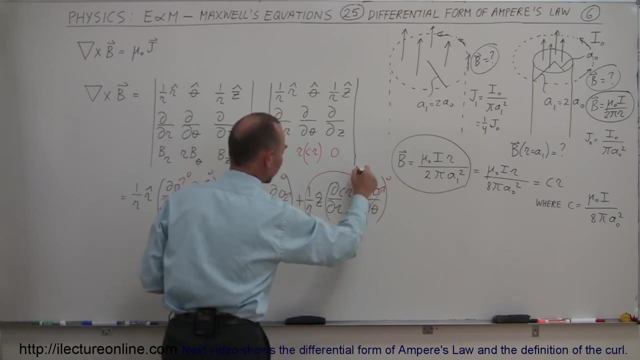 zero. the partial of a constant is zero, the partial zero is zero, the partial zero is zero. and here the partial zero is zero. The only term that survives is this term: right here, that's the only surviving term, not with the negative sign there. all right. 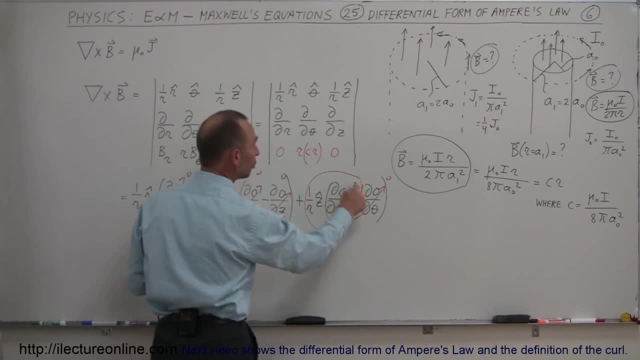 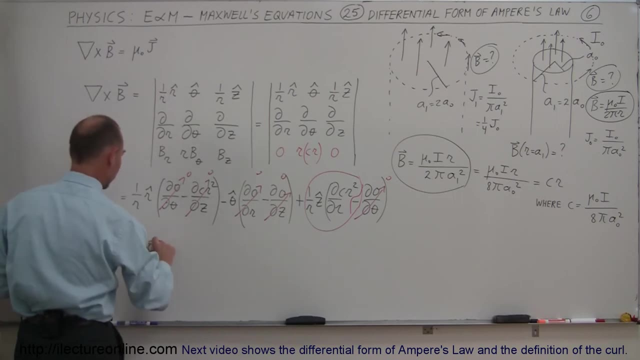 So the partial derivative with respect to r of c r. squared, you'll get two c times r. so this then becomes one over r times z. unit vector times the derivative of that, which is two c r, two c r. 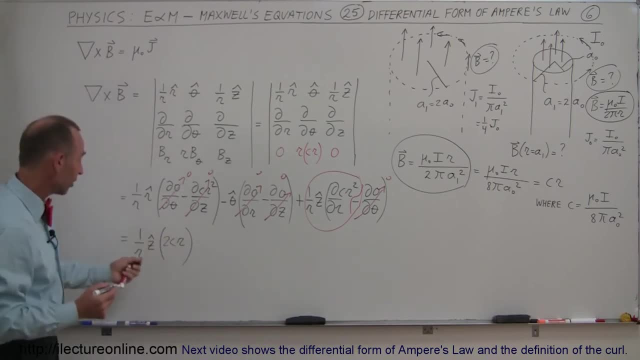 like that. and of course then when you multiply that you get one over r times r, the r's cancel out and you get two c times the z unit vector. Yep, okay, for a moment. there I go wait a minute. z unit vector is there? no, no, because the current 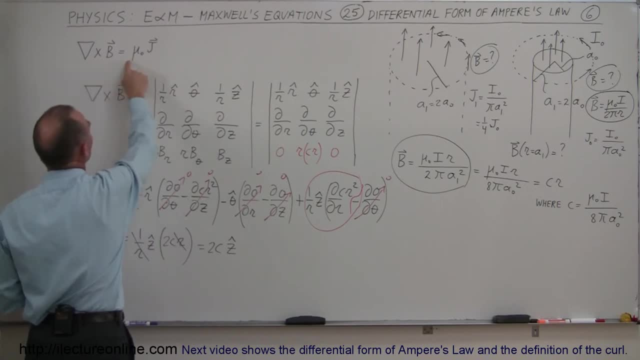 density is in the z direction. so we know that when we take the curl here we should equal. we should equal the mu sub naught, which is the permeability of free space times, the current density in the z direction. so it looks like so far we're on the track of getting the right answer. All right now. 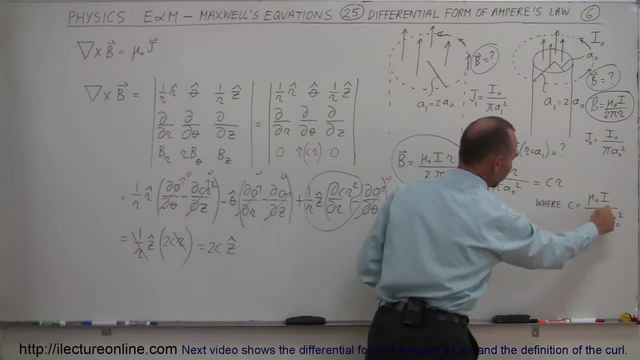 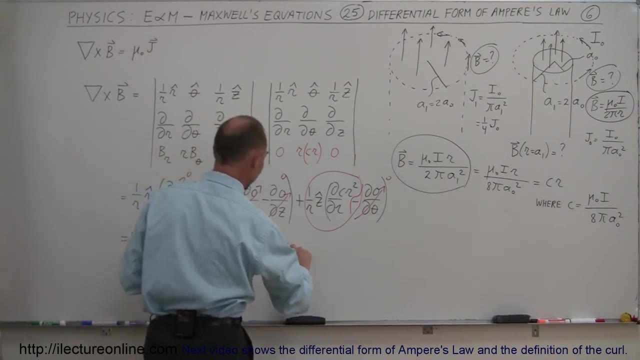 we need to plug in what c is equal to, which we have over here. c is equal to this quantity right there, so we can say that this is equal to r squared, which is equal to r squared, which is equal to 2 times c, which is mu sub, not times i, divided by 8. pi a sub, not squared, of course, 2 divided. 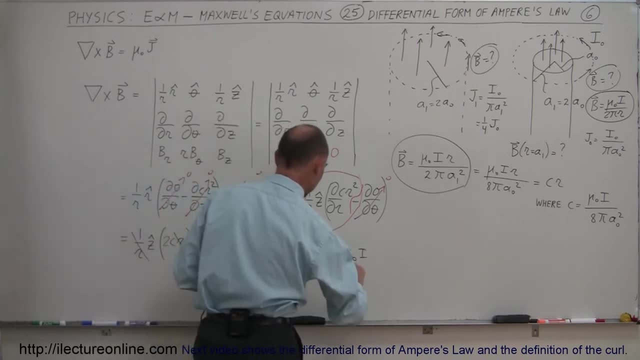 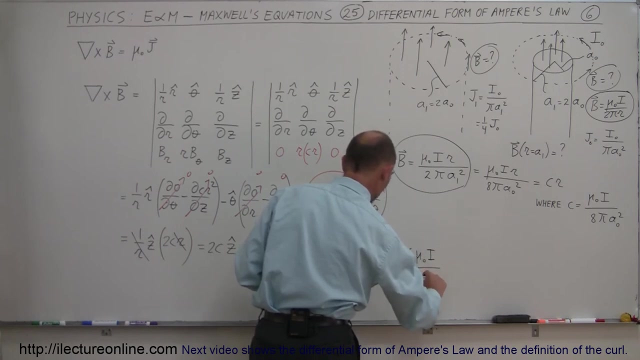 by 8 is one-fourth. so this is equal to mu sub, not I, divided by 4 pi, a sub not squared. and then if we break that out we can say this is equal to 1 half times mu sub, not i, divided by 2 pi in the. 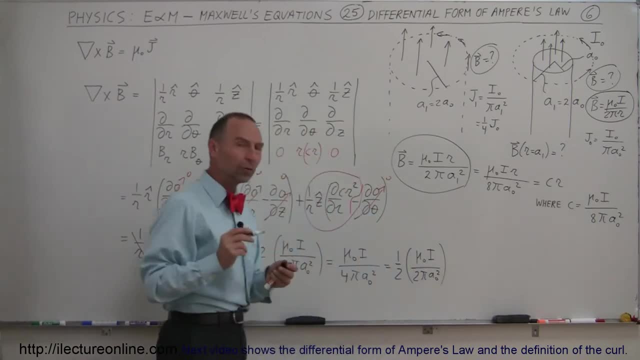 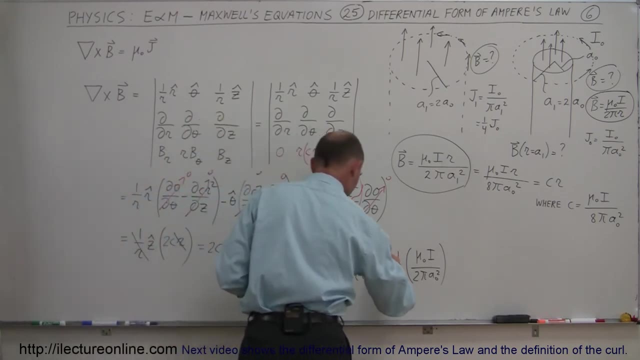 pi, a sub naught squared. so the reason why I wrote it like that is because this portion right here and of course I keep forgetting my z unit vector. I don't want to do that. my z unit vector, there we go. my z unit vector, there we go. and the reason why I wrote it like this is because this portion 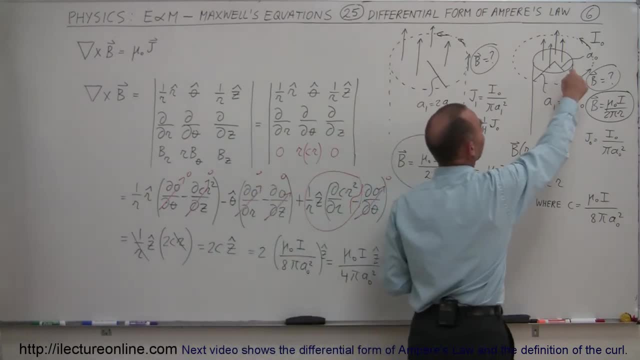 right here is equal to the b field at the edge of the current region right there. so if I find the b field right there, I would get this result right here. but since I now want to find the b field out here, it's only half as much. that's why I wrote all that, so you can see it. at first we would think 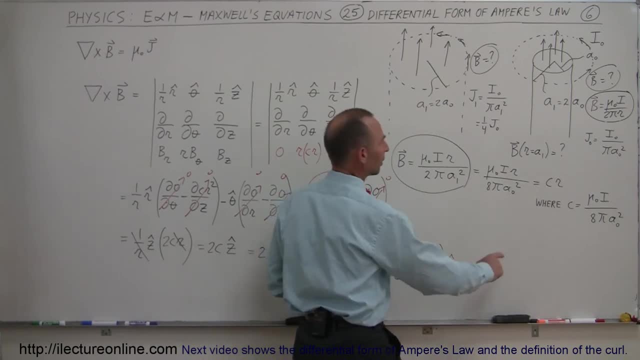 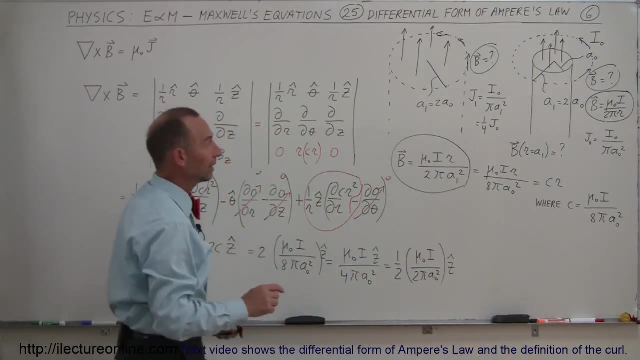 that we got the wrong answer, because here we have an, a sub naught squared, and there we have one over r, and so you say what's going on. but then we have to make one more differential. this equation was obtained by using the integral form of of Ampere's law, and we're using the. 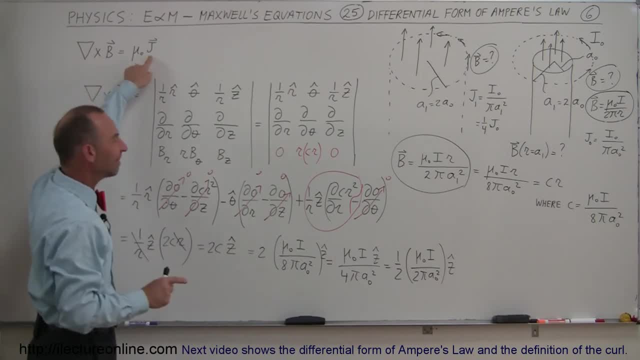 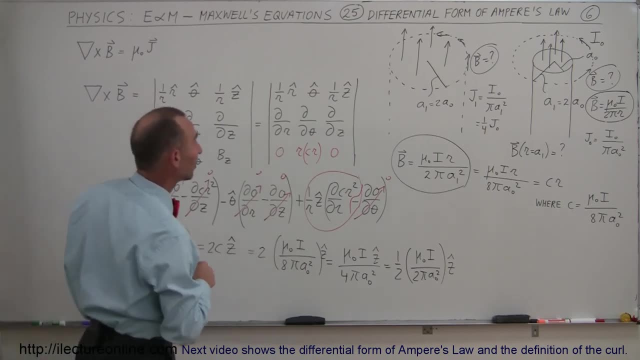 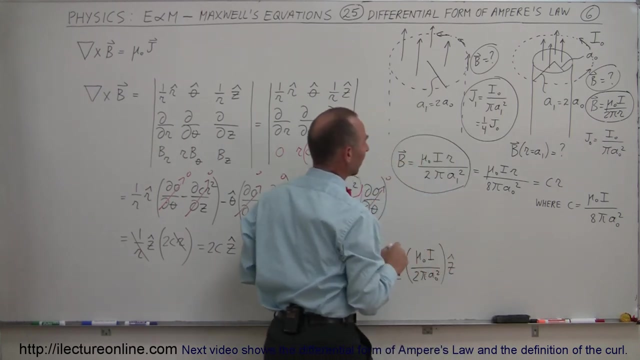 differential form and the curl is equal to mu sub naught times the current density, not mu sub naught times i i enclosed. so what we're going to do is- and I have it here somewhere right here, so I have a relationship between the current density and the current itself. all right, and so i sub naught divided by: 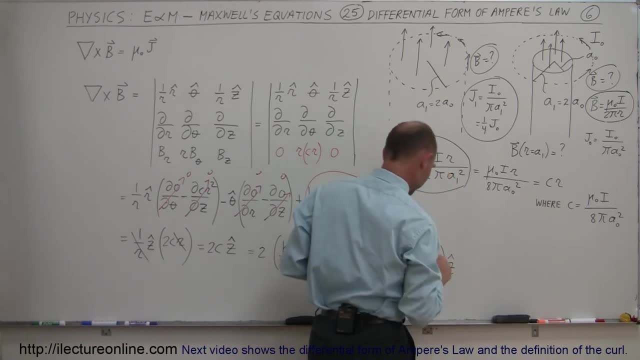 pi a1 squared. we don't have an a1, so we have an a0. so we can write it like this: so we can say that- let me go over here. so the current density j sub naught is equal to i sub naught divided by: 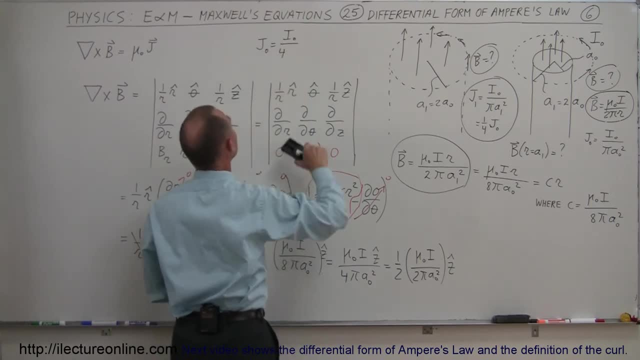 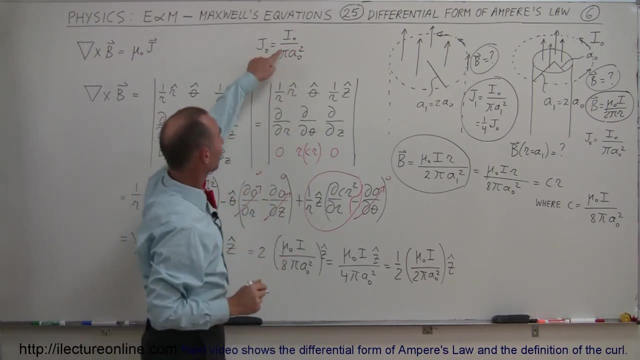 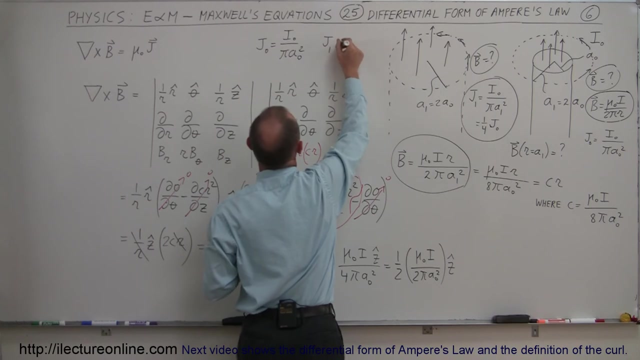 four, not four, because it's area is equal to pi a sub naught squared. all right, so it's equal to the current divided by the area to which it goes. and we can also say that j sub 1 is equal to i sub 1, which is the same as i sub 0 divided by pi a sub 1 squared, which is equal to i sub 1 divided by.